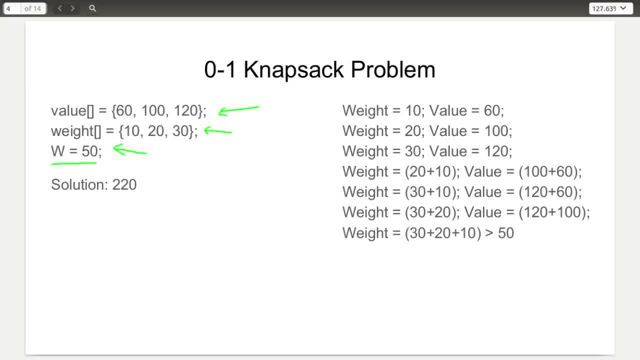 that while we are taking the weight of the item, we are taking the weight of the item and while staying under this weight constraint, we obtain the maximum value. So on the right side I have written all the possible combinations of the items that we can put in the knapsack. 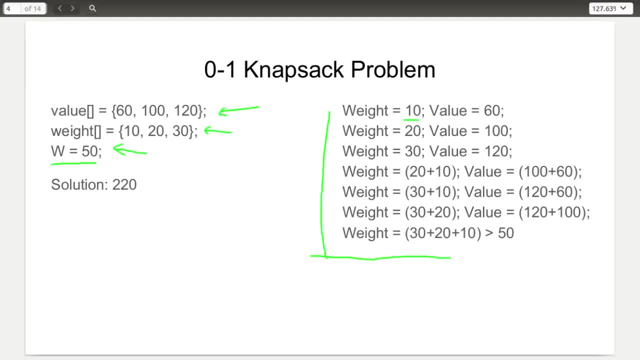 and you can see the corresponding values that they yield for every weight, every possible weight. So, of course, since none of these items are heavier than 50 units, so we can try to put more than two items. So if I try combining items, I see that I get a weight. 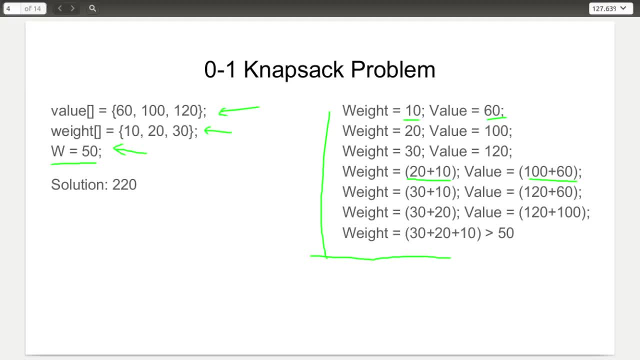 of 120 plus 10. That gets me a value of 160.. So now for weight 30, I have two options: Either I get the value of 120 or 160. So obviously, between these, I prefer 160.. Similarly, 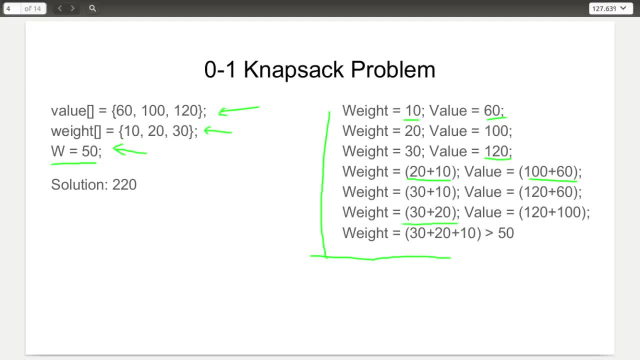 going up, I see that I can get a weight 50 by combining the item with weight 30 and 20 and for this I get a weight of a value of 220.. And I can't put all these three items because they will exceed the weight capacity. 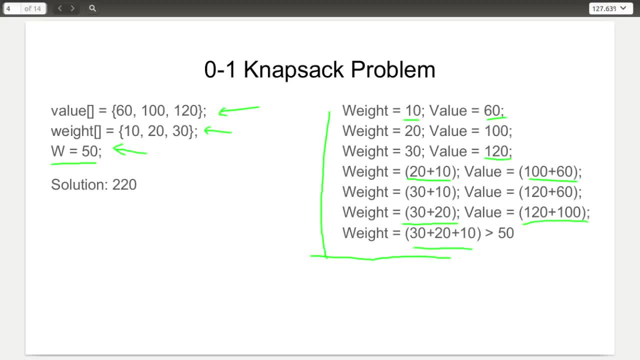 So what this problem means is that, as we keep on increasing the weight, while we do not exceed the weight capacity, we see what the maximum value is that we can achieve. So for this problem, our answer is going to be 220 because, while staying within the 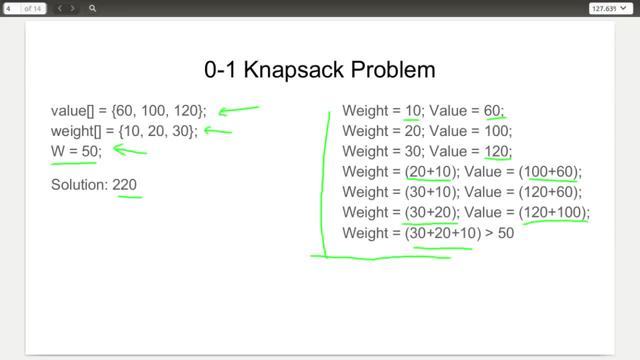 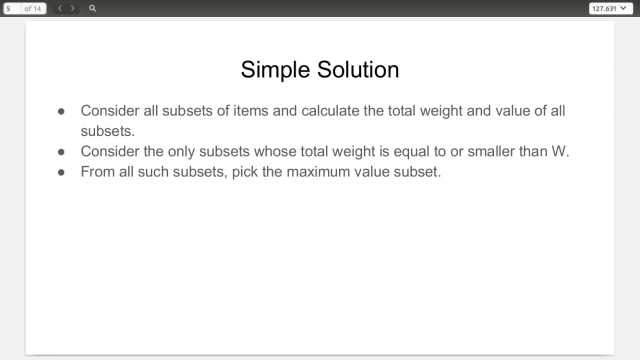 weight constraint of 50, we can obtain the maximum value of 220, because that is the maximum of the six values. So… Let us try to come up with a nice solution to this problem. Let us discuss this nice solution over here. So what we do is we begin with considering all possible subjects of 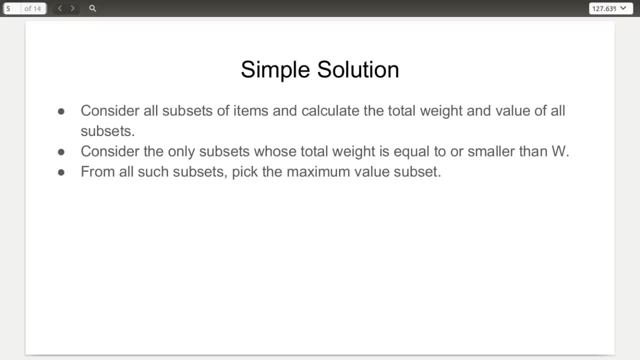 item and we calculate the total weight and the value of all subsets. And once we are done doing that, what we do is we consider only those subsets whose total weight is either equal to or smaller than w. So, and after that, the next step is from all of these subsets. 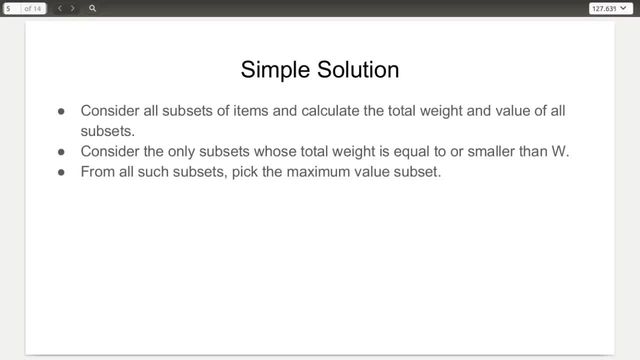 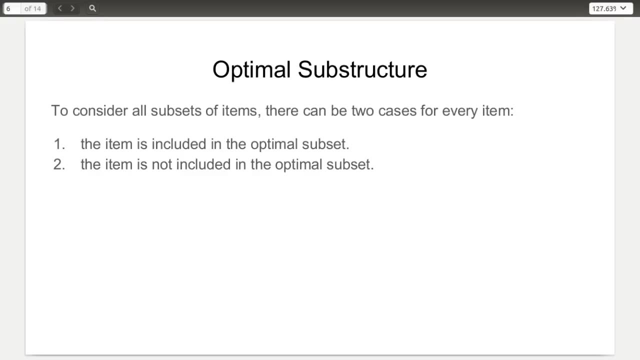 we pick out the maximum value subset. Now, when we say to consider all subsets of items, what we are really saying is, for every item there can be two different situations. Either we include this item in our optimal subset or we do not include this item in our optimal. 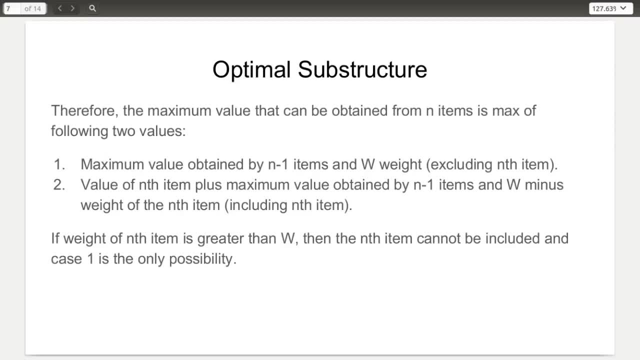 subset. So let us see what this basically translates too. So what this basically means is we have a problem where we are given n items and we want to find out an optimal subset of these n items. So in the beginning we have n items and a weight constraint and we have to do 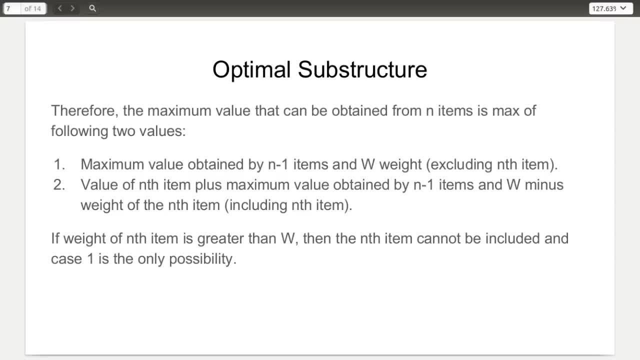 some operation so that we decided whether we can keep the current item in focus in our optimal subset or not. So, one by one, we will consider if we can include a given item item in our optimal set or not. So how do we go about it? So, basically, in order to obtain 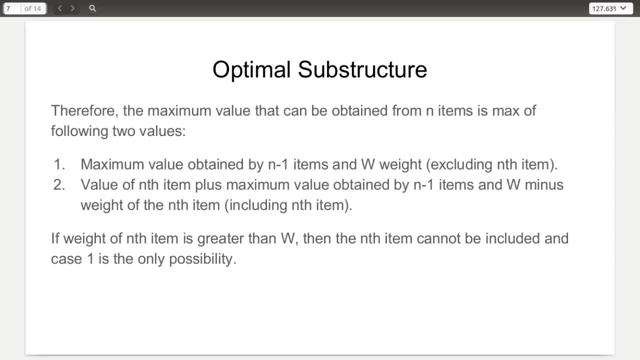 the maximum value. we have to make a choice in the following way: We begin with the reducing this problem to not selecting the nth item and instead moving on to n-1 items, while I mean reducing the problem to that of n-1 items, and the weight remains same. So, basically, 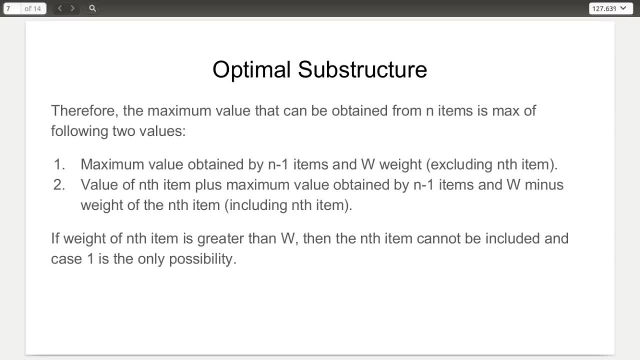 we are considering the case that what if we do not include the nth item and we just solve this problem for n-1 items and w weight? Do we get an optimal value? Do we get a bigger value? And the other case is we take the nth item and then we reduce our problem to obtaining 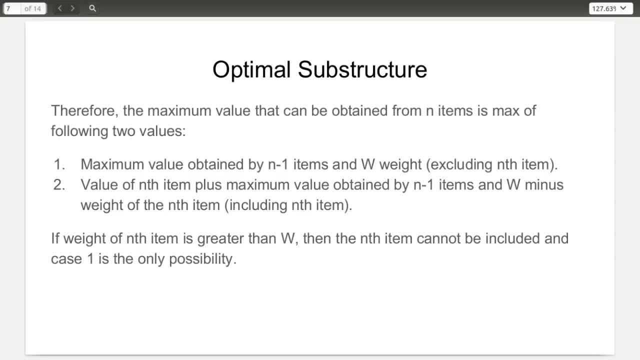 the maximum value of by using n-1 items, but this time we reduce the weight capacity by the weight of nth item and we also count the value of nth item because we are including it in our optimal subset. And we keep on doing this repeatedly until- and we keep on repeating this until- I mean 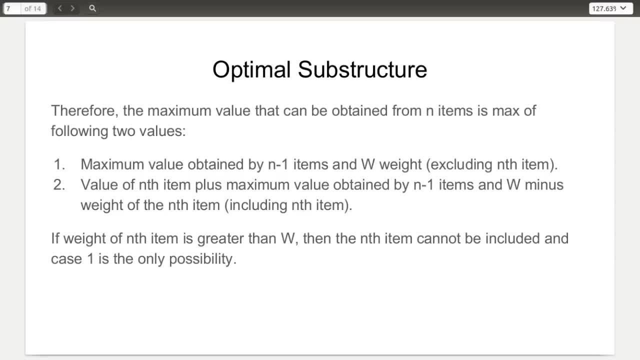 we are not left with any more items. We are done considering all the items. And also there's this thing is, if weight of the nth item itself is greater than w, then of course we can't include it in the optimal subset, which means that we must leave this item and proceed with. 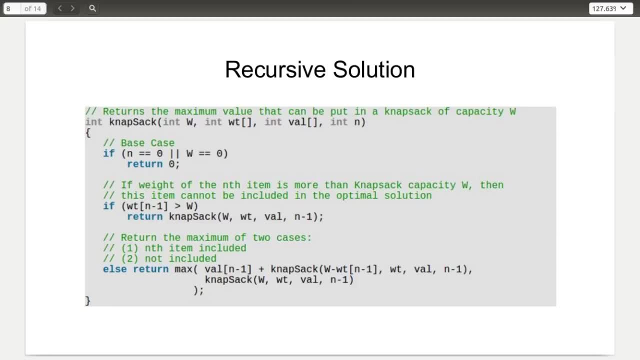 n-1 items. So here is a recursive solution. So let's see what's happening here. We have a set of items which is going to return the maximum optimal value, and this is given the knapsack- weight constraint as a parameter, the weight array, the value array and the 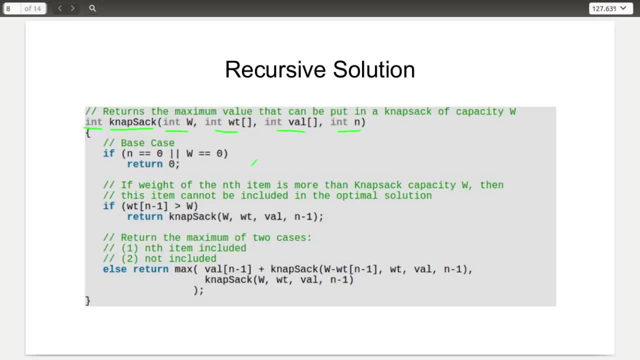 number of items. So, as you can see, we have three cases over here. Now this is very similar to what we just discussed on the last slide. So the case one is: it's pretty straightforward. the base case over here is: if we have n is equal to equal to zero, or weight is equal, 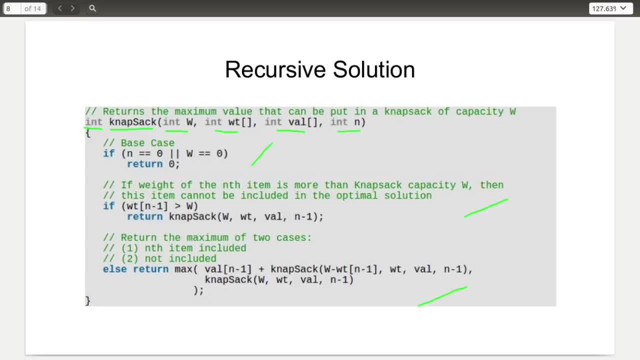 to equal to zero, we return zero. So basically, if we don't have any items to put in the knapsack, we don't get any value. So we return zero. If the knapsack weight capacity itself is zero, we can't put anything inside the knapsack, I mean, unless we have some items which has 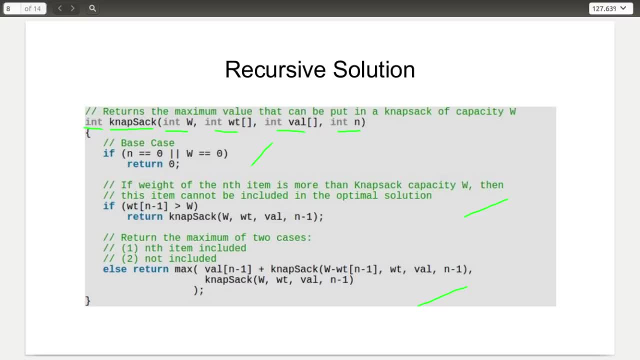 the weight capacity zero, but that's not really a general case. So in either of these cases we end up returning zero. If there are no items or the knapsack weight capacity is zero, we return zero. Moving on, next, we perform this test at this second level In the second. 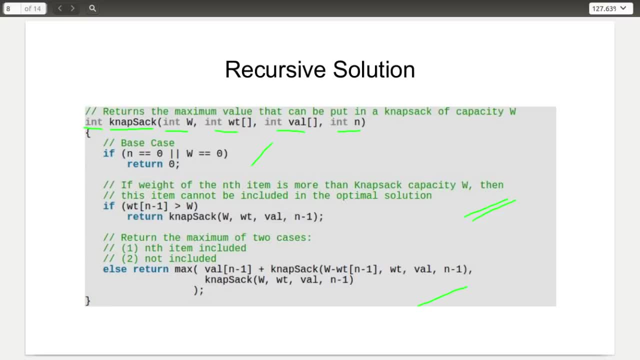 part. So we check if the weight of the nth item- the nth item that we are considering, whether do we include this item in our optimal subset or not. So we check if the weight of this item itself exceeds the w weight capacity. If it does, we exclude it. If it doesn't. 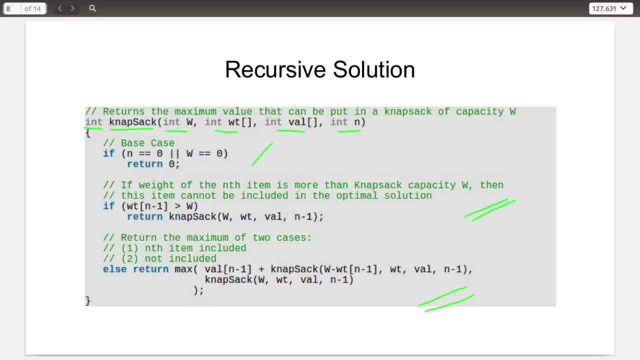 then we move on to the third case. Now, third case is the one where the weight of the nth item does not exceed the weight capacity, And now we want to see if the nth item forms not. So now we make two recursive calls to the knapsack function, In this case over here. 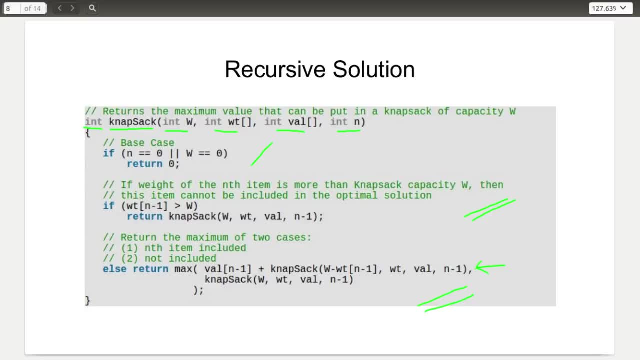 we are including the nth item in our optimal subset and in this case we are not including the nth item. So we recursively call the knapsack function and we wait for the. I mean, we recursively call this knapsack function in these two ways and then, when we obtain their values, we compare. 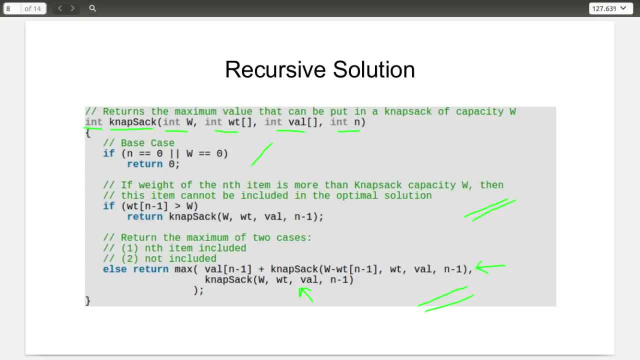 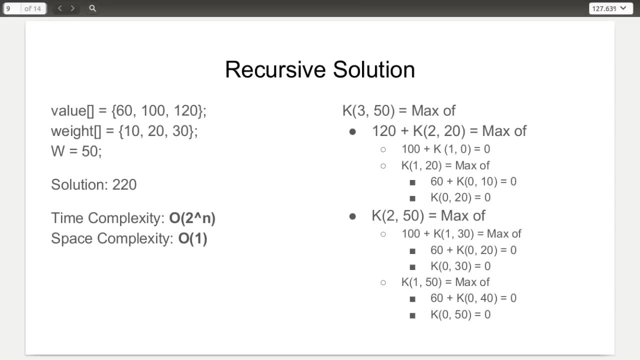 and whichever one of these values is greater, we return that value. So let us do a dry run of that, the solution that we just saw. So we will be using the same example. We have the same weight array, same value array and same knapsack weight. 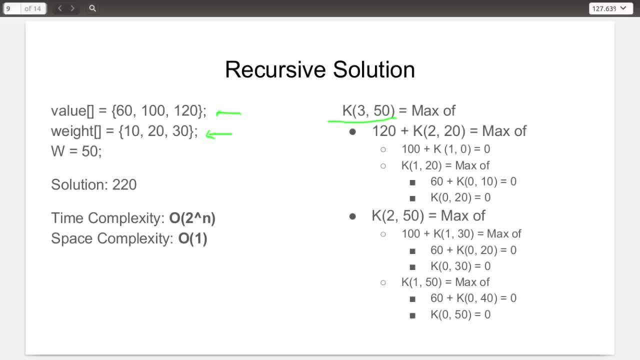 capacity constraint. So we begin with something like this: So k means that we have three items and 50 is the knapsack weight capacity. So when we call k, this problem is divided into these two parts. In case one we consider including the third item. 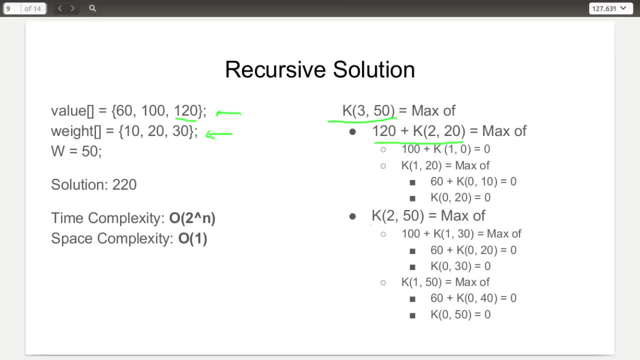 the value of which is 120, and in the second case we consider excluding it. So you can see that when we include the third item, we are accounting for its value, which is 120, and we are reducing the knapsack problem by one item and we are reducing the weight of. 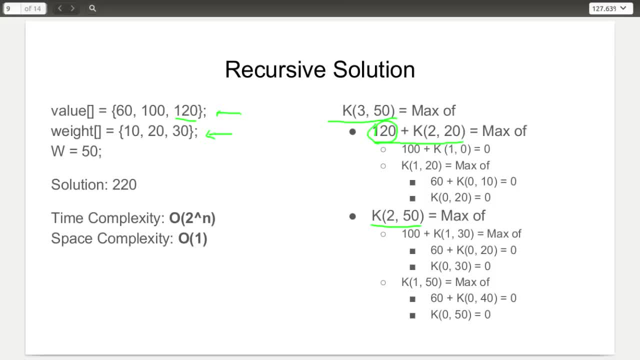 the weight capacity of the knapsack by the weight of the third item. So this becomes 50 minus 30,, 20.. And in the other case, since we are simply including the third item, we reduce the number of items by one and the weight capacity remains same, and so on. 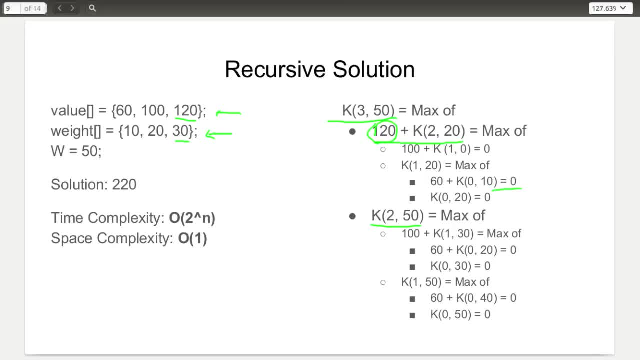 We do this repeatedly until we arrive at a base condition where you know either the number of items is zero or the weight itself is zero, In which case if we return zero, we reach one of those base cases. So, as we see, as you can see later on, I mean so if you, if you take a look at these two. 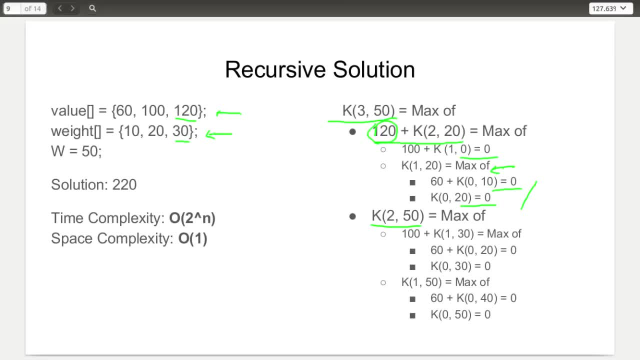 branches. you know that this max will receive a 60.. will receive a 60 and then, if you take a look at these two branches, you know that these two will result in a maximum of hundred. So, basically, K220 will get you a hundred. Similarly, 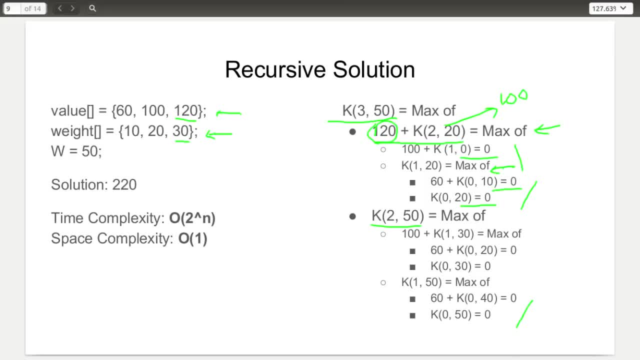 if you come over this side, you can see that if you take a look at these two branches, you see that the max receives a 60 and similarly, this Max also gets a 60, and this Max then gets 160, because hundred and 60 for this Max. However, the second branch is only getting. 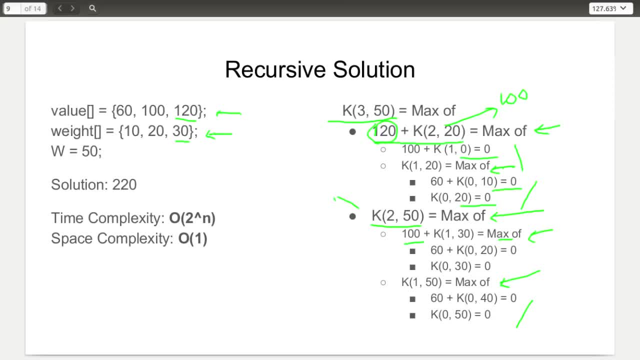 a 60 to 160 is greater in this case. So K250 yields us 160.. So, of course, if we add 120, we get 220, which is our answer. So this is how the algorithm runs. So the time complexity. 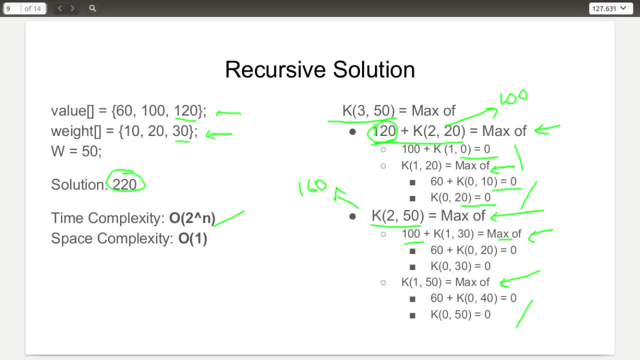 of this algorithm is going to be. we go off two days to end because we have n items and for every item we are making a choice: whether we increase or decrease. So that's how we get the same complexity And since we are not using any extra space, 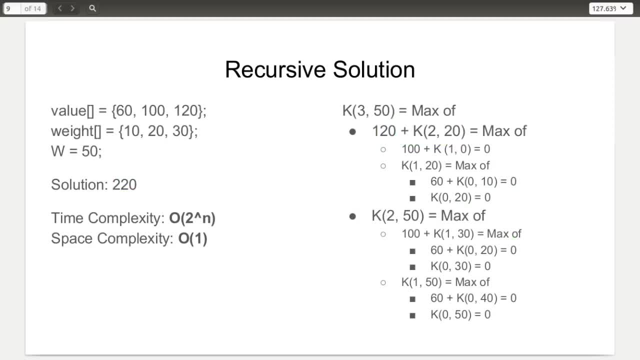 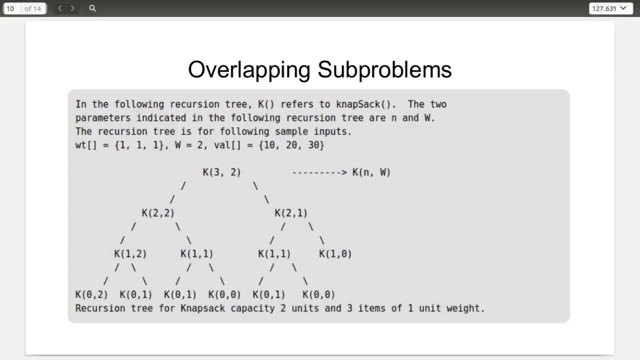 so our space complexity stays big of one. Now there is this interesting thing that you can see here is if we, if you call the knapsack function in this case, this is another example where we have three items, All of those have the same weight and the values. 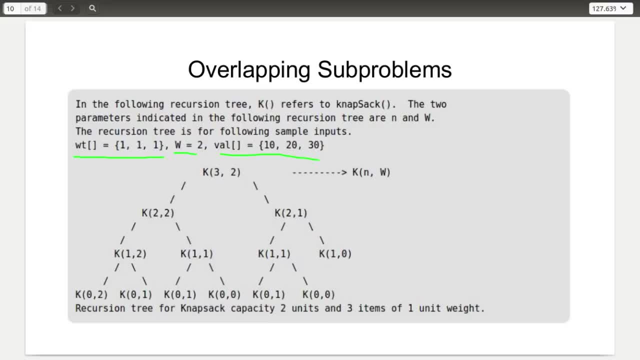 are 10,, 20,, 30 and the weight capacity is two. So so in this case, as you can see, we begin calling the knapsack function with the parameters three comma two. three is the number of items, two is the weight capacity, And you see that on both of the sides. So 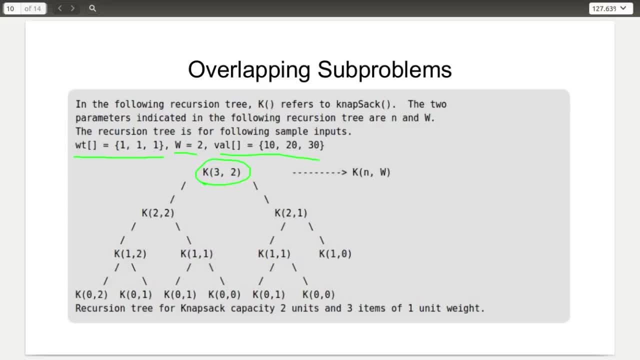 at every step, you see that the tree is divided into two parts. The left part is when we include the nth item, and the right part is when we include it. So, so this is where we include the nth item. This is where we include the nth item, and this is repeated for all the 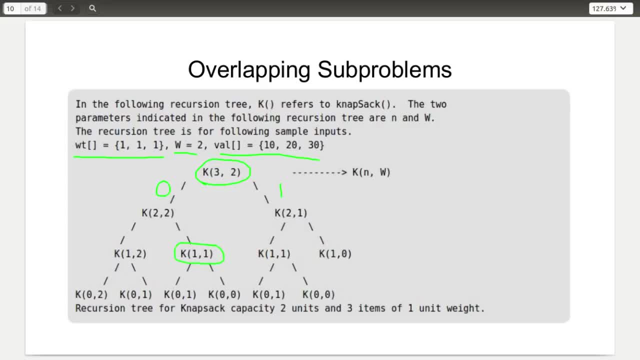 subtrees. So if you look down here, you see a K comma, K one comma one appearing over here, and a K one comma one appearing over here too, And so so this means that we are solving the same problems on both the branches, And if you further look down, you'll see that this 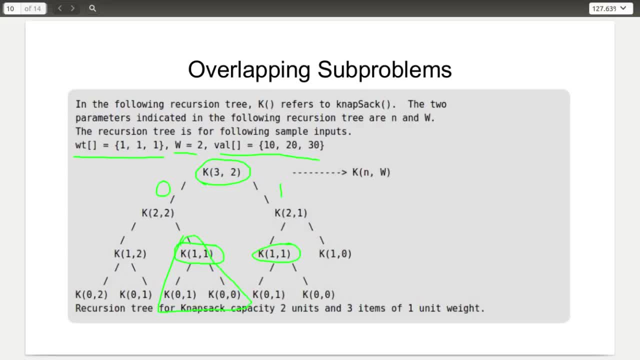 whole sub tree is actually repeated, Sorry, So. so this is a very small example. I mean, uh, for a bigger example, we can see that there will be a bigger subtrees and all those computations will be unnecessarily repeated. So so what we see here is that we have a 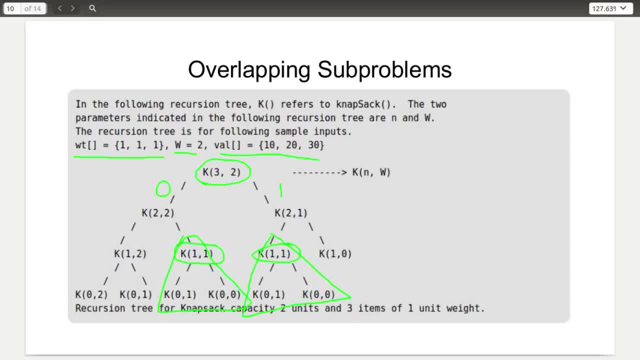 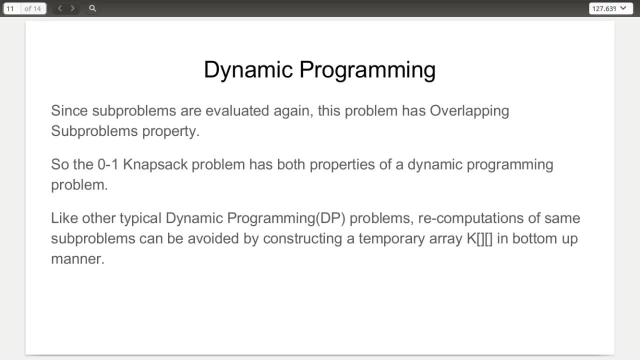 number of subtrees. So what we see here is the uh like this knapsack problem satisfies the overlapping subproblems property. So since now that we have seen that the zero by knapsack problem satisfies the overlapping subproblems, a property, and uh so, and it also has. the So so uh, now uh. so we can see that. we have seen that uh, the0, 1 Knapsack problem satisfies the overlapping subproblems property and uh so uh, and it also has the. 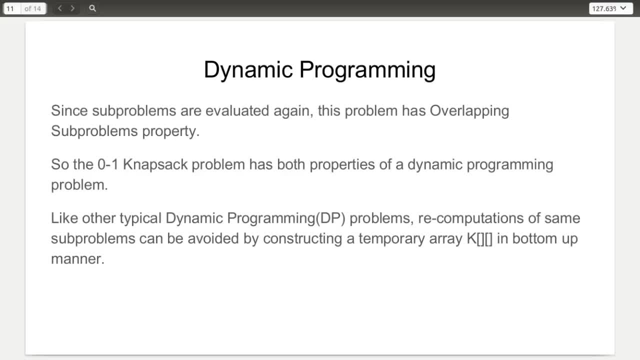 the optimal substructure property. So optimal substructure comes where we repeatedly solve the same problem. So you saw that we were changing the parameters of the knapsack function and yet we were recursively calling the same function again and again and arriving at a solution. and then we also saw that some of the problems were overlapping also in different 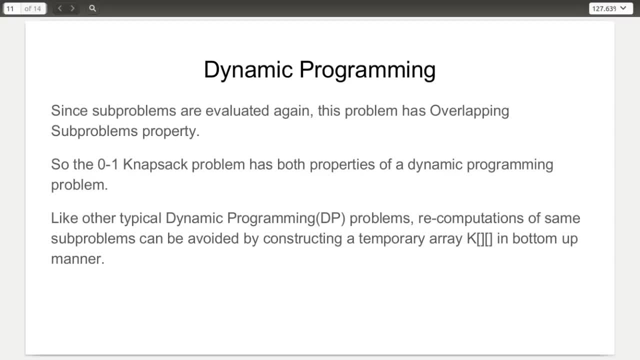 branches. So this makes the zero one knapsack problem a dynamic programming problem, because a dynamic programming problem is anything that has the two properties: the overlapping subproblems and the optimal substructure. So let us see that if we can come up with an algorithm where we avoid all these computations of the same subproblems, and maybe we can build 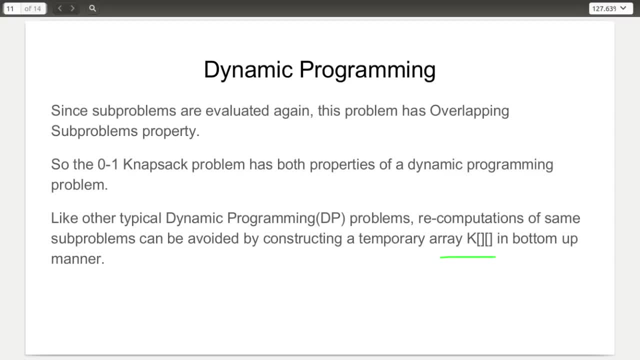 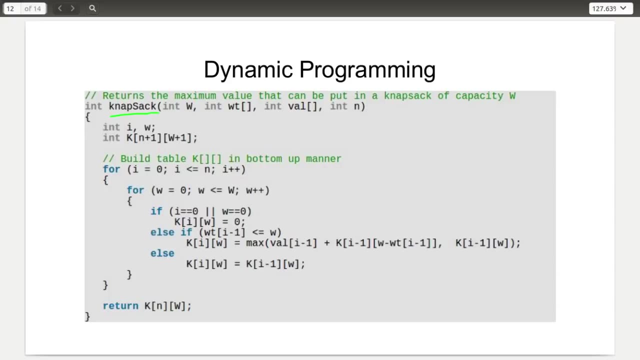 a temporary array in a bottom up manner and then we can just look up the values for problems that we have already solved. So we don't solve the same problems again and again. So here is the dynamic programming approach. So we have the knapsack function over here and you 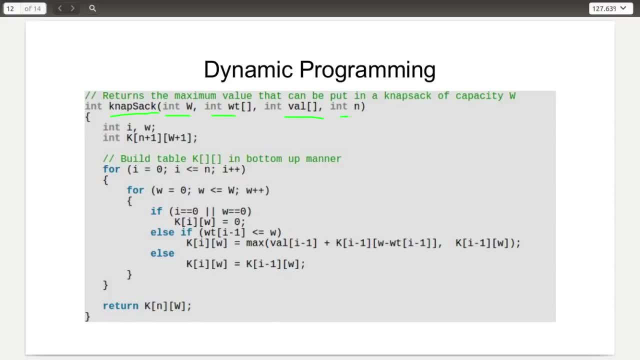 have the weight capacity, the same weight array, the value array and the number of items. Now we have this n plus one into w plus one dimensional array. Now this is where we are going to store all the solutions. So whenever we solve a problem and say we solve k one, 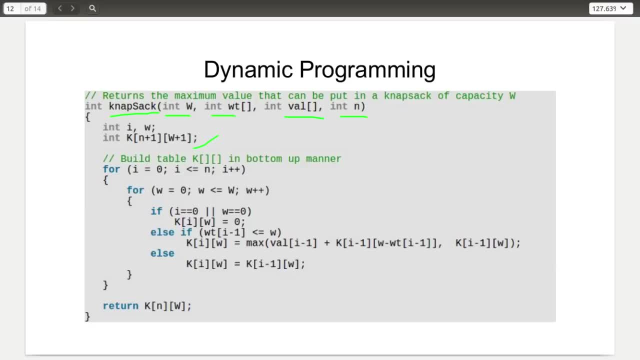 comma zero, or we solve k zero comma one. So we will put the solutions and the values that we obtain: Okay one comma zero. Sorry for the bad handwriting. So so if we have solved k one comma zero, we will just update the value of k one comma zero as zero, and so on. So, moving on, we will. 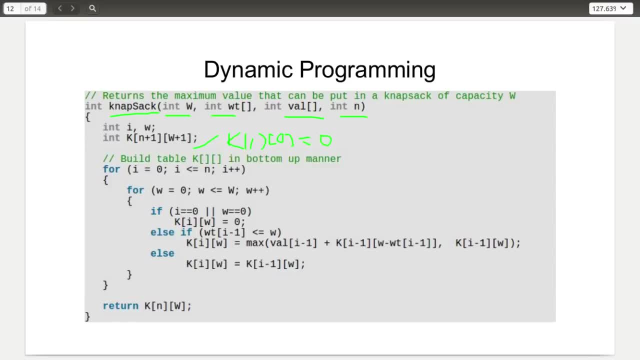 follow a bottom up manner, and at every step we will update one cell of the this k matrix, and this is how we will eventually arrive at our solution. So so we have two loops over here. The first loop runs n times and the inner loop runs w times. So the first 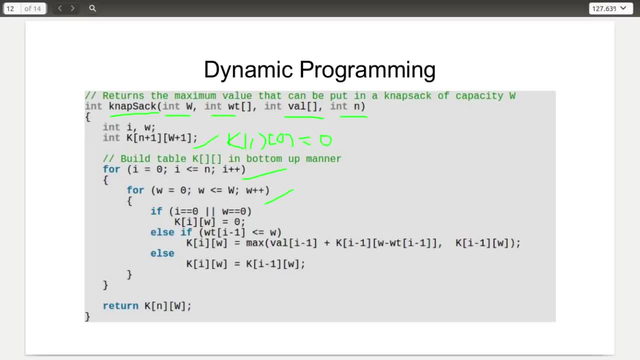 loop is simply to show that we are considering one by one all the items. and the second case is considering the case where we are trying out different possible weight scenario and we are finding the solutions to these combinations and we are storing them. So in the inner loop, 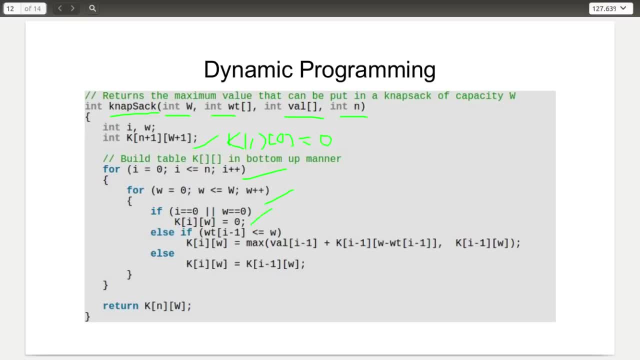 we see that if i is equal to zero or the weight is zero, So basically, if the number of items is zero or the weight is zero, we know that the solution was to return zero. So we are simply storing zero in our matrix. So all. 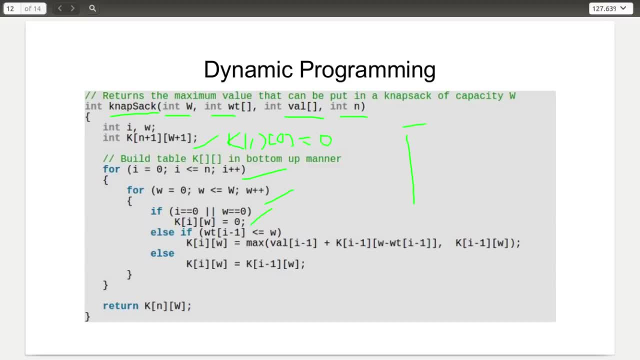 the k zero comma w, or all the k w comma zero, The first row and the first column of our k matrix are going to be all zeros. So moving on, in the second case, we so here. now in the second, if we check whether the weight of the ith item, which is for the given problem, the nth item I mean, 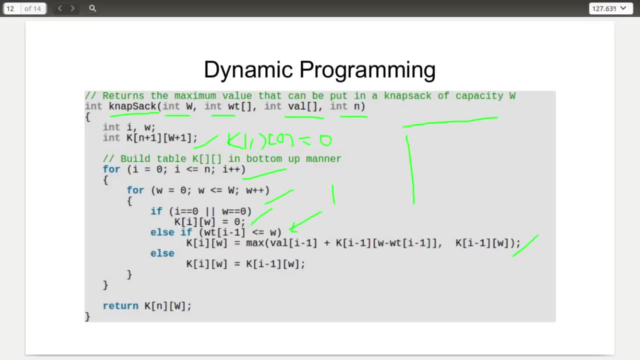 if so, so at every step of this loop, what we are really doing is we are solving this problem: K, I comma W, So, so, so at every iteration. what we are really doing is we are considering whether we should be including the ith item in our optimal subset or not. So the first 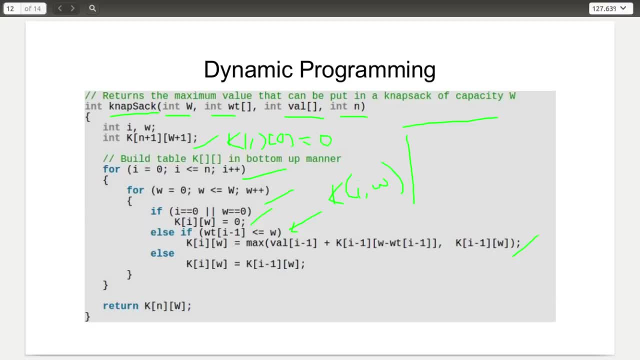 thing that we are doing is we are checking whether the weight of the ith item is exceeding the knapsack weight capacity or not. If it's not, then we move on to the optimal substructure solution part as so as if you remember from the recursive implementation or from the earlier, 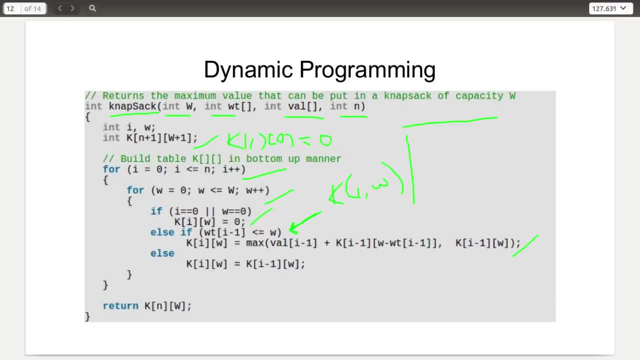 discussion that we had about the structure of this problem, the solution. So we saw that whenever the weight of the item is not exceeding the capacity, we make a choice. we consider two cases. case one is when we consider including the item and case two is when we think of 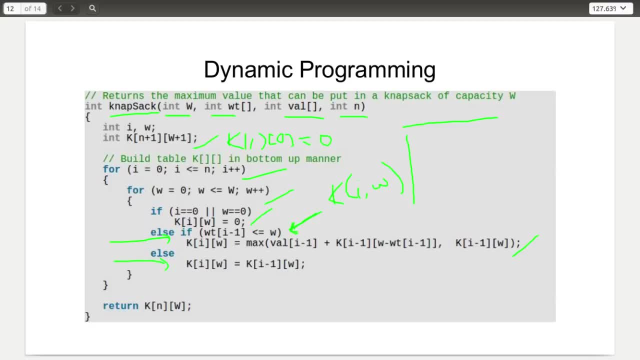 excluding it, and we see what we get. so now here. so now here, if the weight of the i-th item does not exceed the capacity, what we do is we make a choice. so here we are calling the max function with two parameters. now, parameter two is okay, I a minus 1 comma W. so this is where we are simply including the NHI. 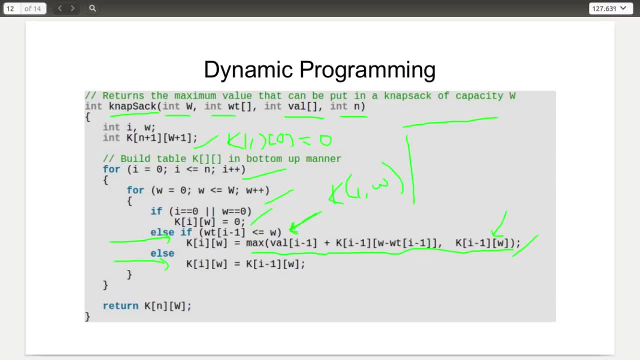 item. and we are just seeing that. what if we include the an ioth item? do we get a bit better value? do we get a better optimal solution? and over here on the left we have an image, as will decir scopata, you can see, is we are considering what happens if we include the item. So we count, we add,